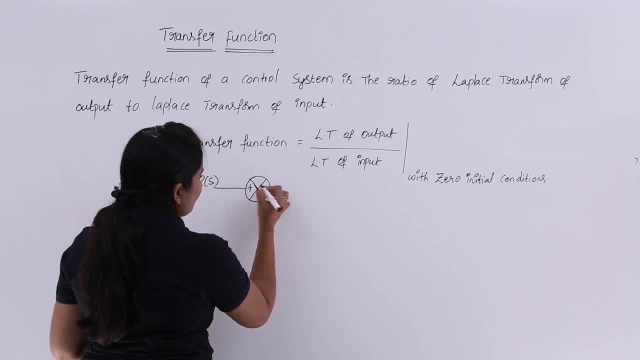 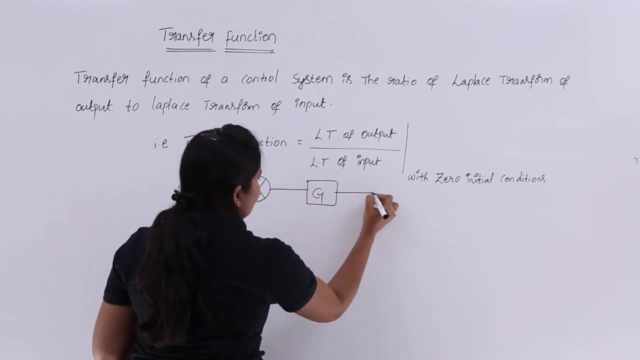 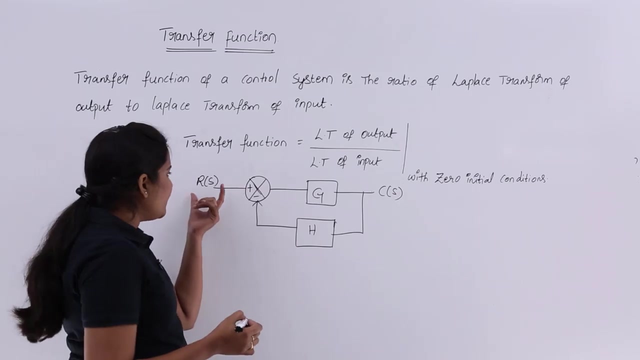 I am having a summer here, So I am having a negative feedback system like this, and here this is my open loop gain G and this is my output transform and this is about my feedback. My feedback gain is H, feedback element gain is H, So this is my closed loop control system here, where 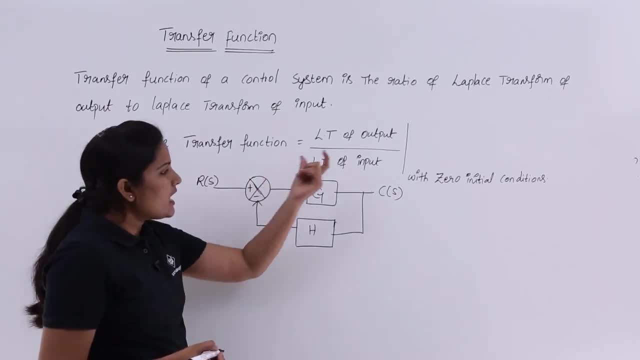 input is R of t, where the input transform is R of s and output is C of t and the Laplace transform. 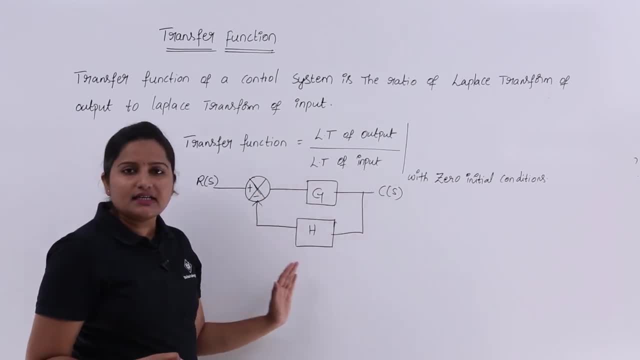 c of t is c of s. so everything i consider in terms of frequency domain and gains. so here, in case of this system, this is a negative feedback system in case of this system. so if you want transfer function, so you need to get by using c of s, by r of s, you need. 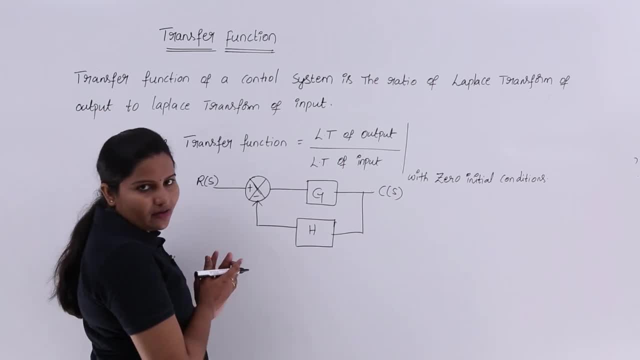 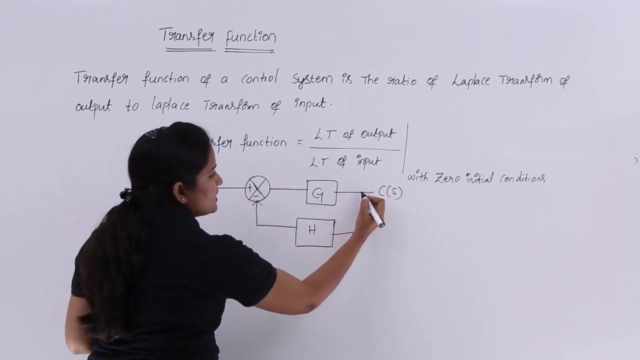 to get c of s by r of s. so how we can get c of s by r of s before getting c of s by r of s or transfer function, i want to get the value here. so here you can see, this is r of s minus c of s into h. so this is the point of c of s, so c of s into h. so i am considering. 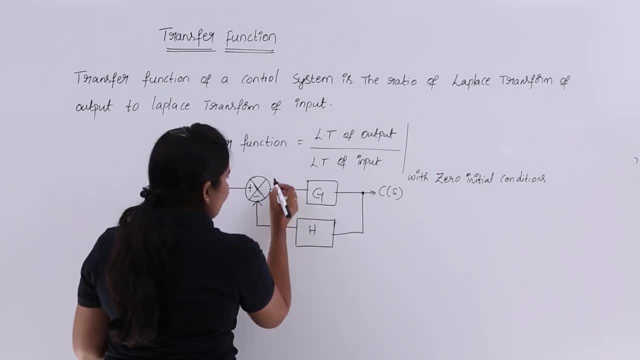 like c, h or c of s into h. so this is the point. so here this signal and the feedback signal. feedback signal is nothing but h into c of s, so h into h, into c of s, so r of s minus h into c of s, so h into c of s, will be the value at this point. 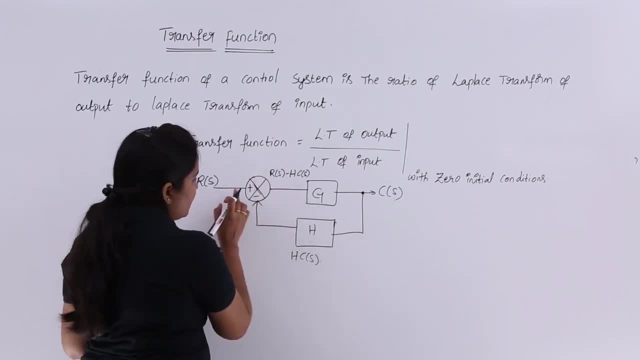 output at this point output. so r of s minus h into c of s, the gain, where h is the feedback loop gain and c of s we are taking as feedback with a gain h. so here the value at here is equivalent to r of s minus h into c of s. now if you want to write the equation, 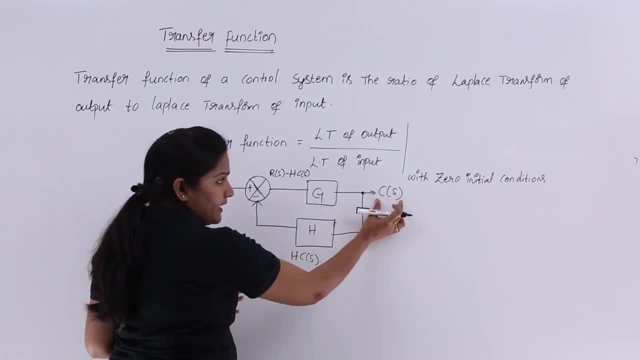 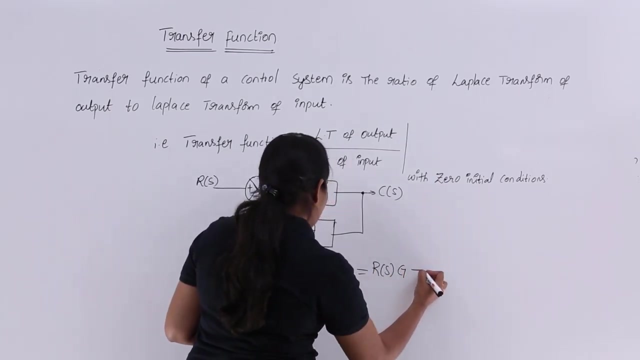 for the output at present point. so the c of s is equivalent to r of s, r of s minus h into c of. here I can write this as: R of s into g, R of s into g minus g, h into c of s, g h into c. 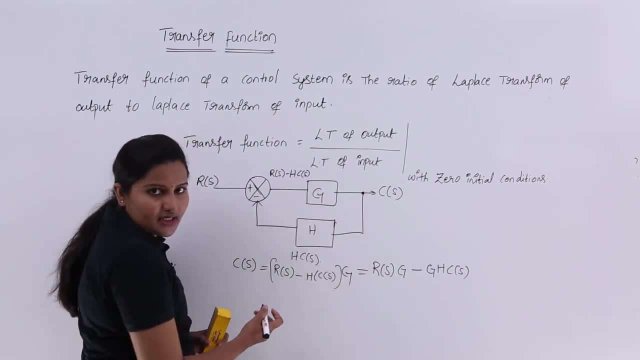 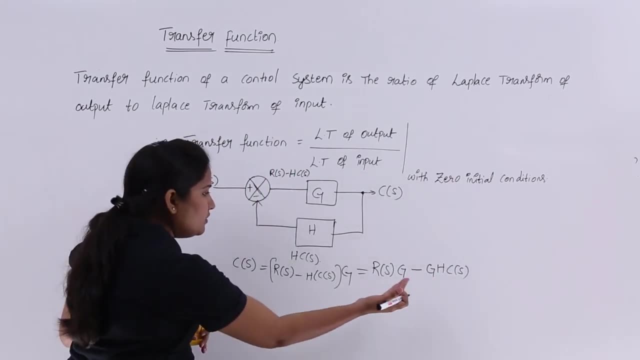 of s. I am just multiplying to inside this g. I am multiplying to inside. Here I am having c of s, another c of s I am having here, So now I can take that c of s to left side, So I will get. I can take common of c of s 1 plus g. h is equivalent to R of s into g. But to 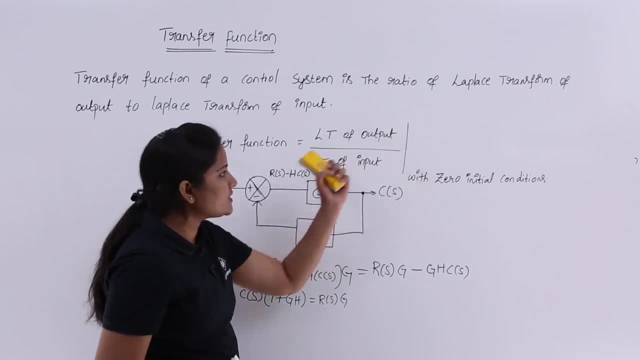 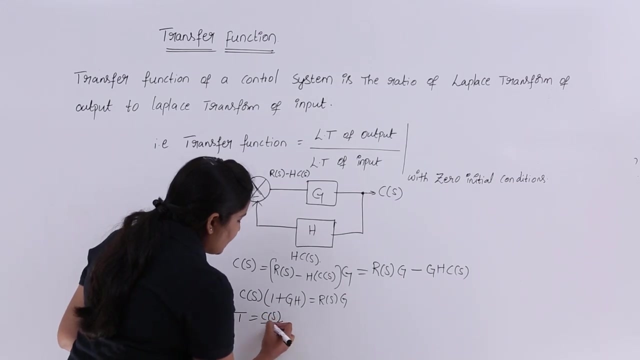 get the transfer function. the equation is: Laplace transform of output by Laplace transform of input. The Laplace transform of output is c of s. Laplace transform of input is R of s. to get transfer function t you need to get c of s by R of s form. So if you send, 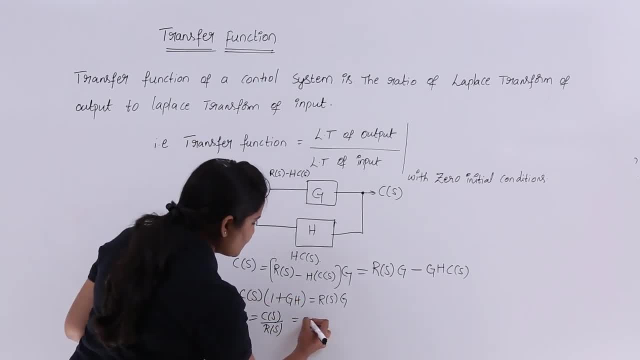 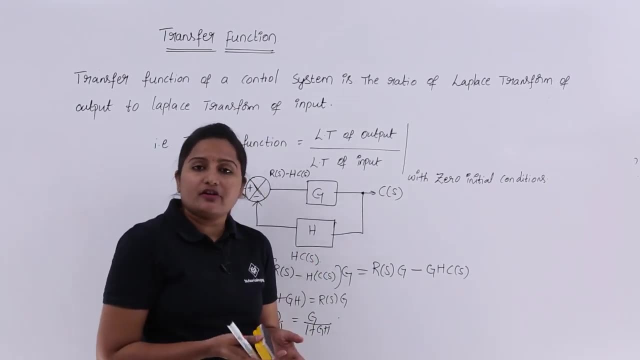 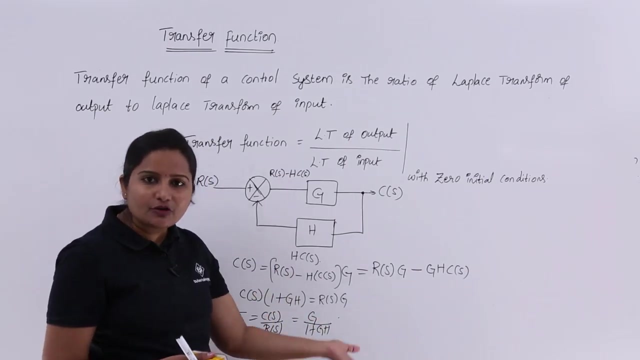 this R of s to this sub unit. You are going to get the transfer function of the system like this way: you need to calculate for positive feedback system also. So maximum we are going to prefer negative feedback systems. So g by 1 plus g, h will be the transfer function of negative feedback system. So like this: 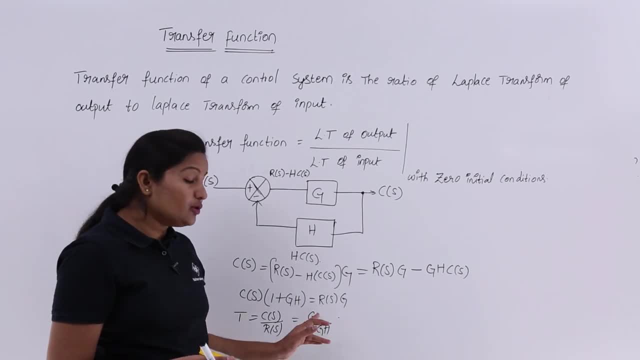 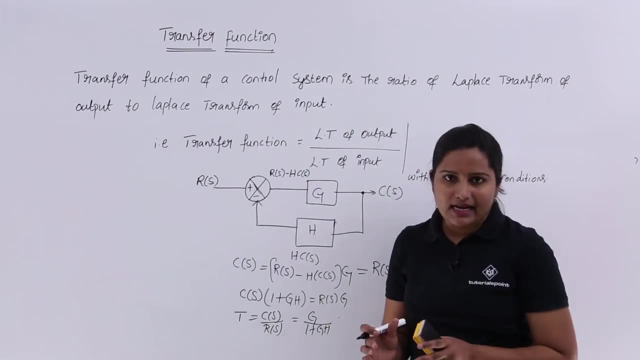 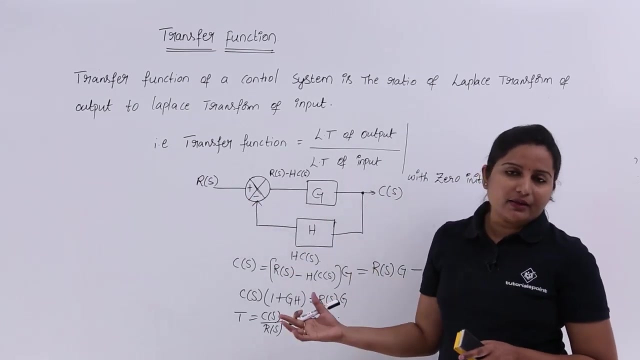 if you calculated the same for positive feedback system, you are going to get g by 1 minus g, h. So this is about transfer function of the system. in the next class We will see how many types of feedbacks are there. So this is negative feedback system we are having. 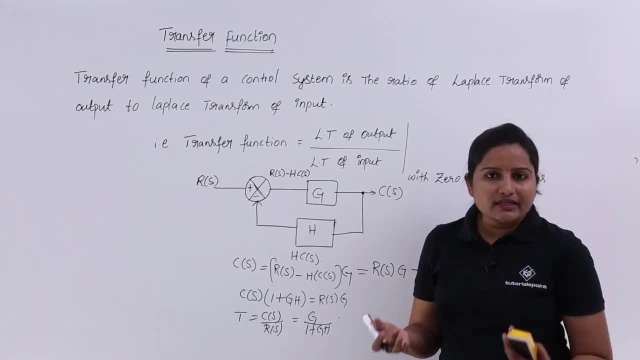 positive feedback. also In the next class we will see how many types of feedbacks are there, How we will write the transfer function of that positive and negative feedback control systems. So we will see clearly there. So this for negative feedback system, the same. 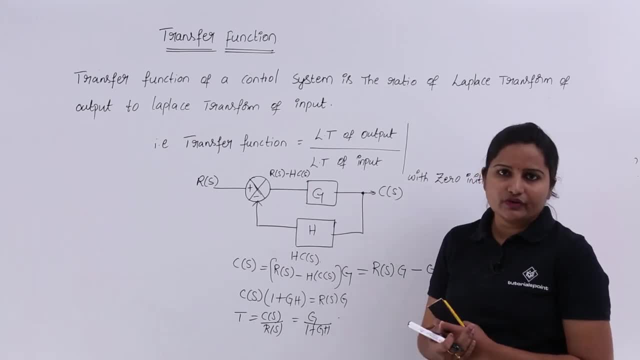 we are going to derive in the next class, also along with positive feedback system. So here the transfer function is nothing but the ratio of output to output. So this is the transform by input transform. In case of control systems. we are going to prefer our output.